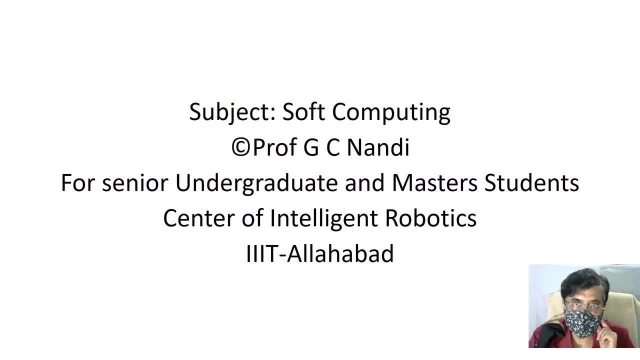 Hello, dear, welcome back. So, as you see, I came from outside and wearing a mask, So please always put a mask whenever you go out. And we are living in a very critical situation. as all of you know, the global pandemic of coronavirus is actually engulfing everybody, So be safe. 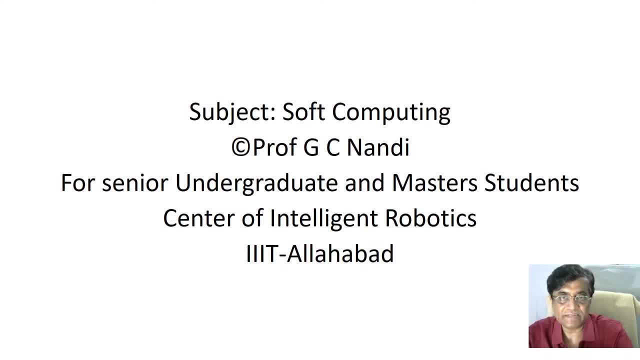 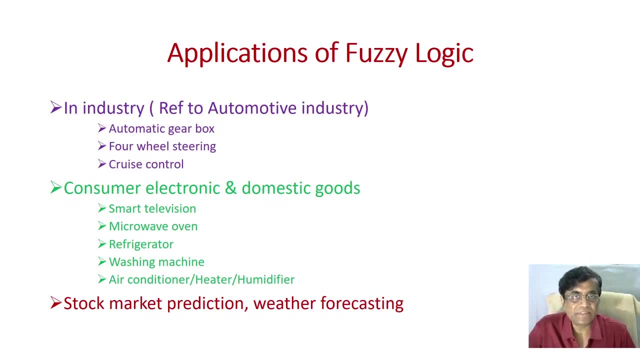 Okay. So with this message now, as we, as I, promised in the last class that I will talk about applications of fuzzy logic. There's a huge application everywhere. almost Okay, But before doing that, I will tell you a small story. Unfortunately, you see, in 1960s, right. 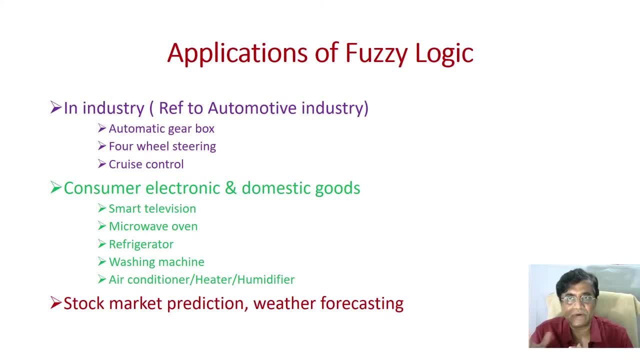 Look, actually he wrote paper, influential paper, and is considered to be father of fuzzy logic. When all these things are happening, many scientists in the and practitioners in the Western world they thought they some sort of undermine fuzzy logic, because perhaps the fuzzy term was there. 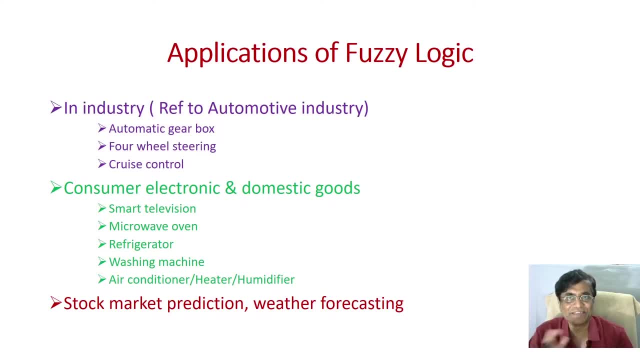 They may be misunderstood that it is the logic which is fuzzy, Not fuzzy logic is the logic which can capture the fuzziness of the environment. So that thing was realized by Japanese people and many scientists, you know, you know and many other reason. I already discussed his inference system So they could realize the true potential of fuzzy logic and a number of 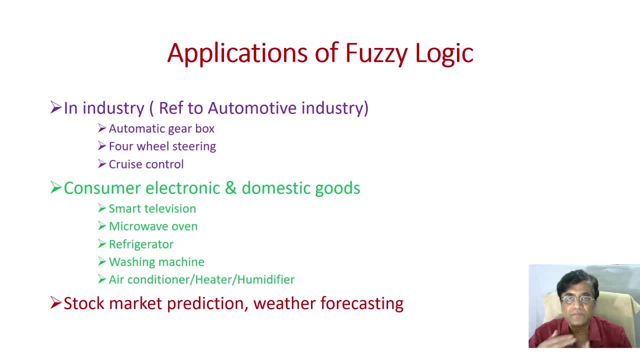 products were developed, Everything was going on, And then in the Western world also, they realized, and then things took a very dynamic state. So today I'm going to discuss, as I promised, that application of fuzzy logic. it has a huge application in industry. For example, automatic transmission, automatic gearbox. You know that you have paid some money and bought a car which has automatic transmission. 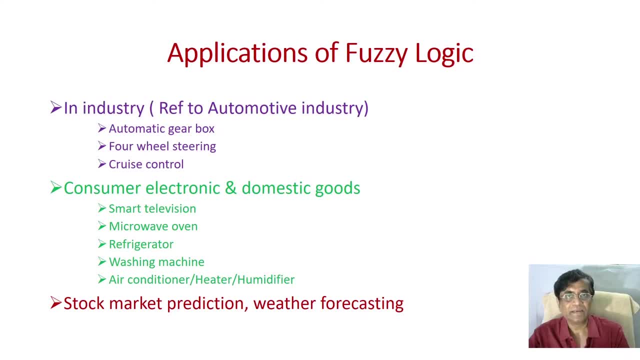 That's all. you do not know that. what is the technology behind it? Only thing is it is giving you comfort not to put stick and slip gear right. So, behind the scene, fuzzy logic is working actually. So it is analyzing that based on, say, your car is climbing a stiff hill right, So you need to lower the gear right, So automatically s e has to be done. 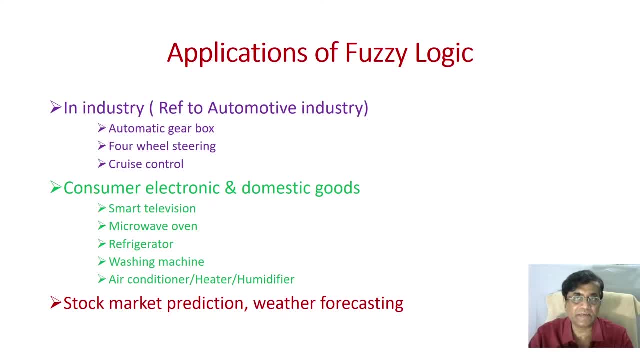 know, but there's a logic. together with the actuating and control devices and sensory devices, it is actually doing that. so in automatic transmission. similarly in four-wheel steering: okay, so you have four-wheel drive, especially when it is snowing right, so so that your car will not sleep. 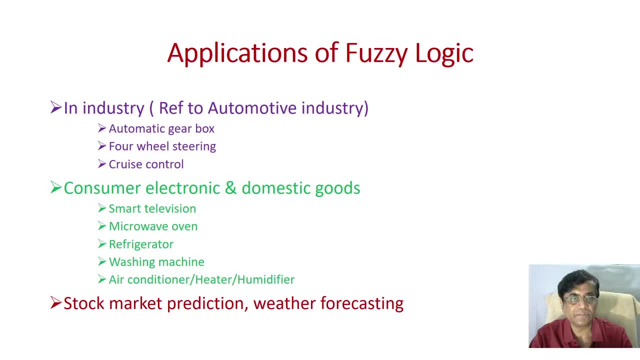 you need to have control. four-wheel drive control is there then quiz control? freeze control is another um modern feature of any automobile, right? so that is there. say, you are riding a car and comfortably at 60 miles per hour speed, you press the button cruise control, so it will try to maintain the same speed. and now suppose the car is going downhill, right? 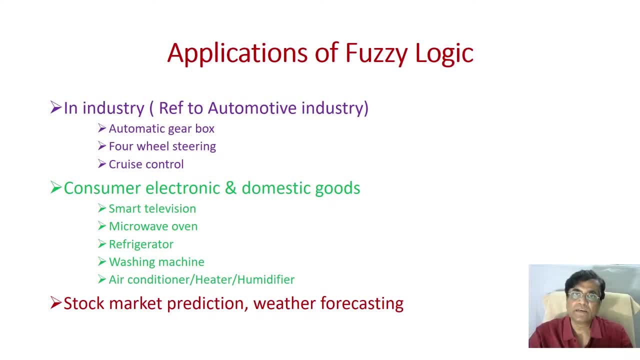 so speed will tend to increase. so there is a sensor, and then fuzzy logic is there. so Sensing, that fuzzy expert system will adjust the fuel injection of the car so that less fuel is injected and then speed is reduced. okay, All kind of, then, consumer electronic and domestic goods. nowadays, this is smart television. 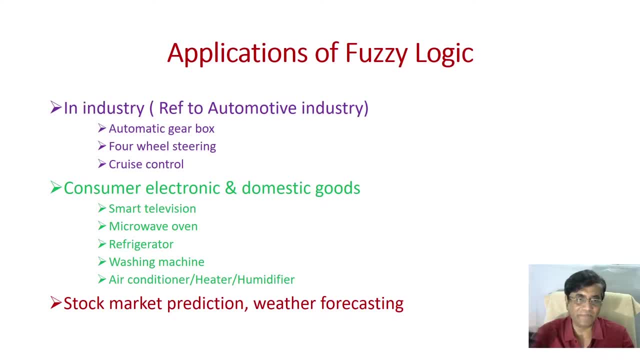 microwave oven- fuzzy chip. is there refrigerator- fuzzy refrigerator. is there washing machine- fuzzy washing machine. is there, fuzzy chip. and I think every household has this kind of thing, air conditioner. So, depending on, or humidifier, depending on the current, if the room temperature is high. 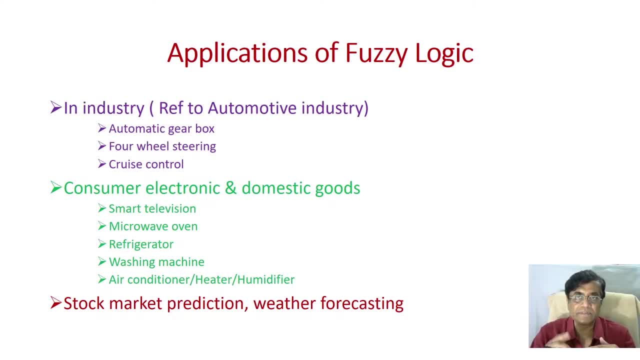 then the temperature you are setting, say 20 degree. so accordingly the compression needs to be pumping out heat from your room and it should run longer, rather than when you set it already temperature is near to your desirable temperature, it should not run. So all kind of logical inferences can be drawn by fuzzy logic. 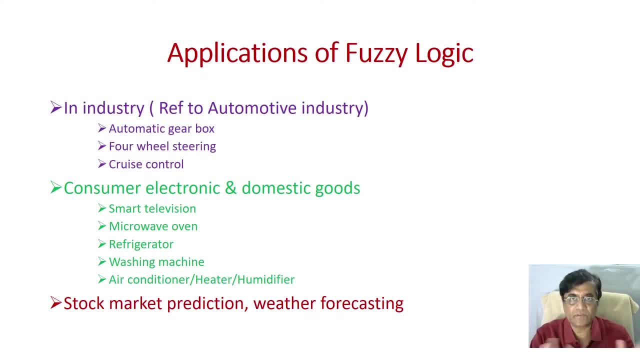 Another stock market prediction, weather forecasting, so everywhere. almost fuzzy logic now it is used. Now, having shared all this, you see I am planning. I am going to discuss how to design a fuzzy washing machine using Shigono approach. okay, 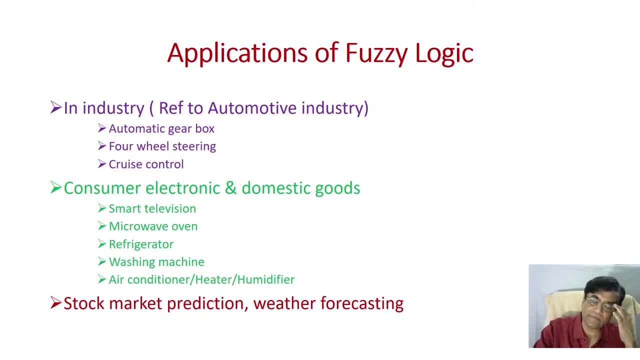 So let us try to. in designing that, I will use a expert system: shell. You know what shell is? shell is just like empty architecture. it is analogous, to suppose, as we have also discussed in my next lecture. Okay, So what we are going to do is we are going to create a new office and nothing is there. 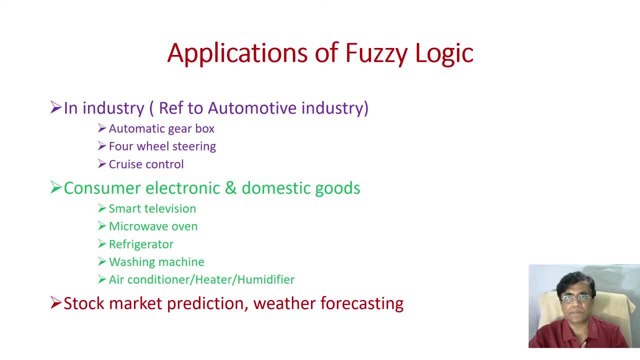 no furniture, no other equipment and all kind of things. This is you who will actually furnace the office. right Empty office is just like shell. okay, So we have an expert system, shell. many open source experts in shell are available and I am using, since we have. 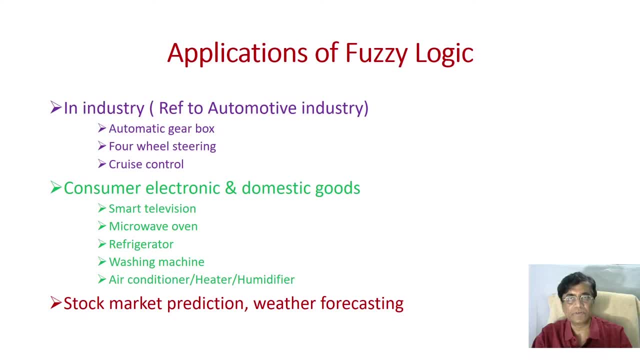 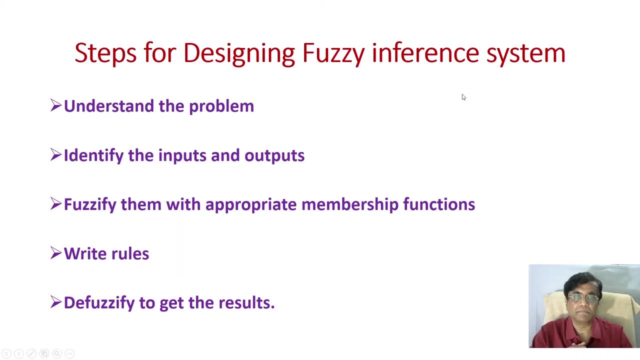 So we are using expert system shell, fuzzy, expert system shell of MATLAB. So in the command prompt if you just type fuzzy, then you will get expert system shell and I will try to use that for designing a fuzzy expert system for mad lab. 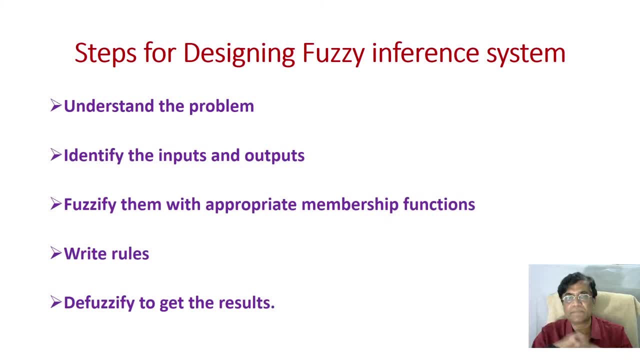 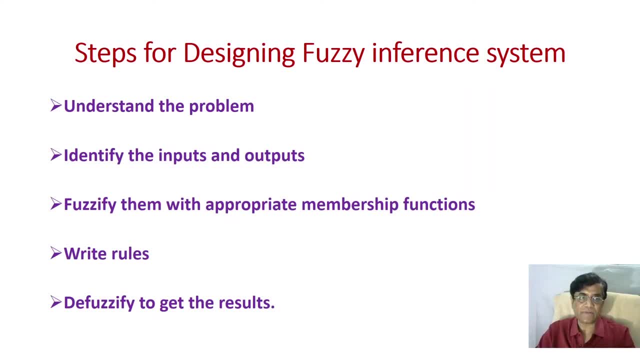 with appropriate membership function, then you need to write rules, because very carefully, because here only you are Capacitate, Capacidade, Capacidade, capturing the actual knowledge. If you write bad rules, performance will be poor. If you write very efficiently rules, then performance of your internal system will be very, very. 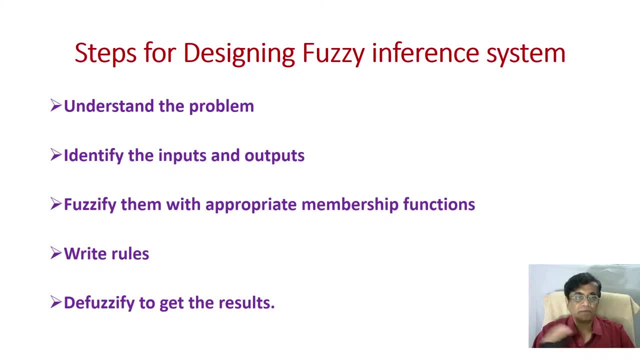 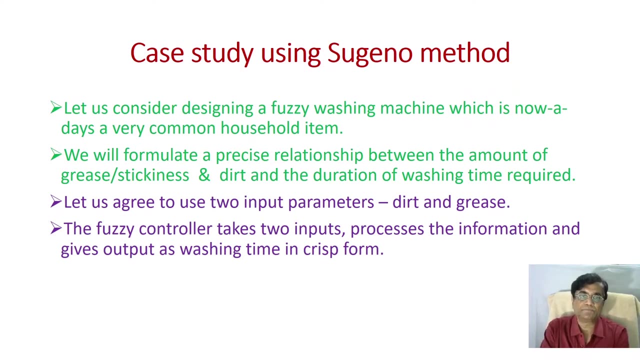 accurate, Then you aggregate when the rules are fired, as we have talked in my earlier lecture, you aggregate the outputs and then you defunctify it to get the result right. So we are doing the case study using Sugano method. We will design a fuzzy washing machine. 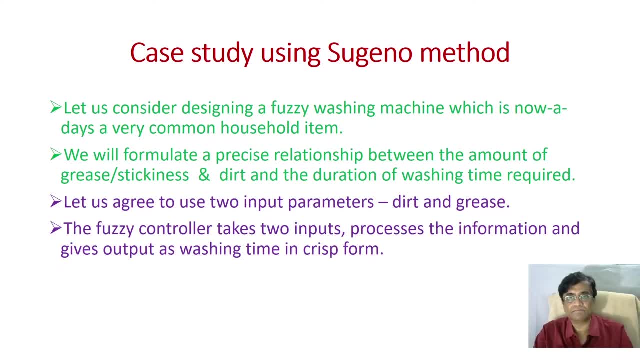 fuzzy chip which will be installed in a fuzzy washing machine so that, in a very optimal way, it will consume less resources and give you maximum output in terms of removing the dirt and the grease or stickiness or oiliness from your dresses. Thank you, 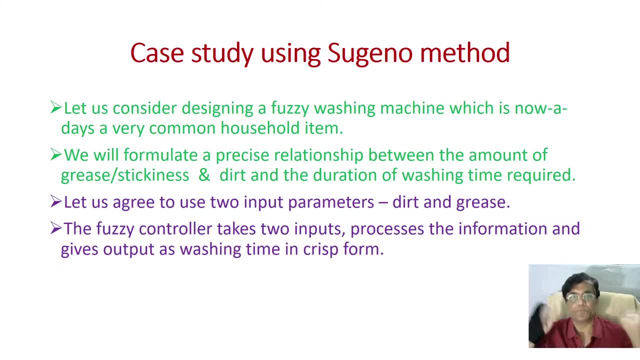 So for that, let us identify two inputs. So this is in your hand. Now you are in the designer seat, So you are the boss, right? The way you will select the parameters, the way you will select, write the rules, the way you will get the result. okay, good, or? 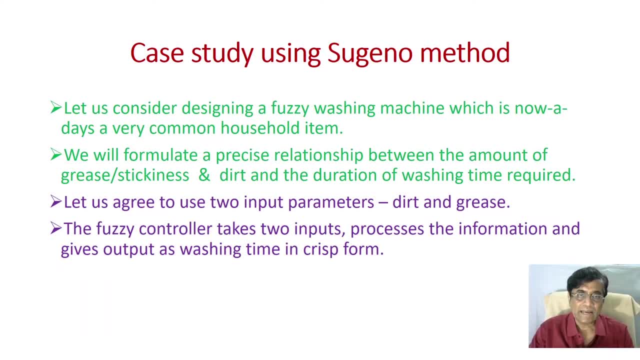 bad. And let us also see that the output is actually two inputs are. two inputs are: one is the level of dirt that is in the cloth or dress and one is the level of the skew that is in the dirts right. 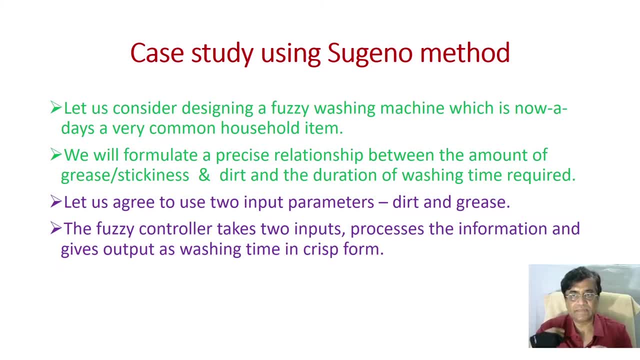 So these are the two things which I decide my fuzzy system should process to give me the optimum output. What is the optimum output? The fuzzy controller actually must tell me washing time, Okay, How much washing time is required, Okay, And then are the buttons. 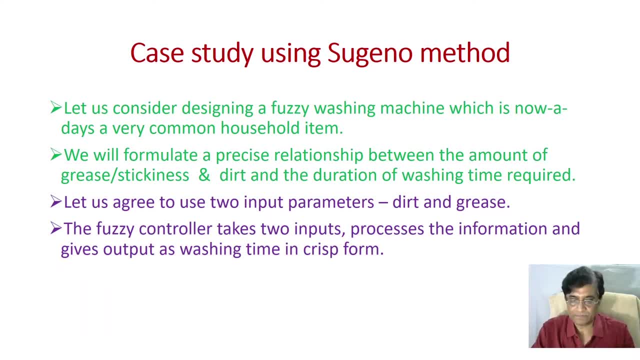 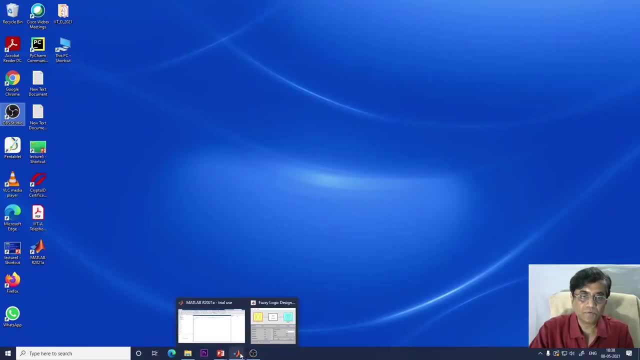 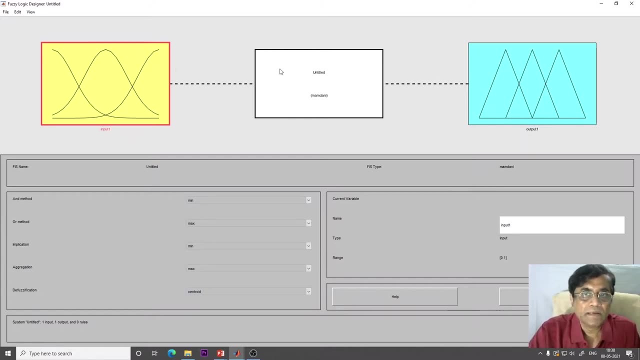 there, Okay, And then you use the control and the control is there okay. So you are time I should have optimally okay. so I will just now try to see, as I told you that I will. this is my expert system cell, so by default, mangani approach is. 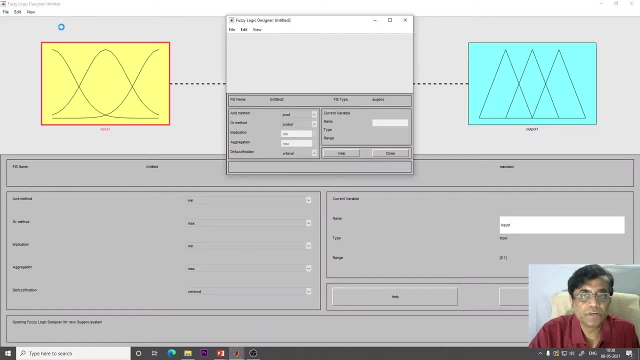 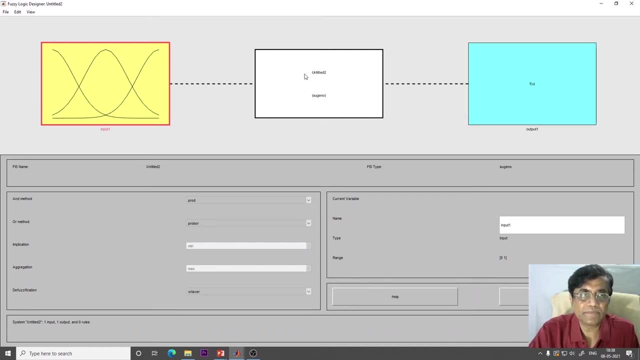 coming. so I told that I will use sugar, not approach. so I have now a sugar, no type of expert system. so as a system I am designed, you see, now I will have to add variables. right input. so how many inputs? two inputs, right, I have decided I. 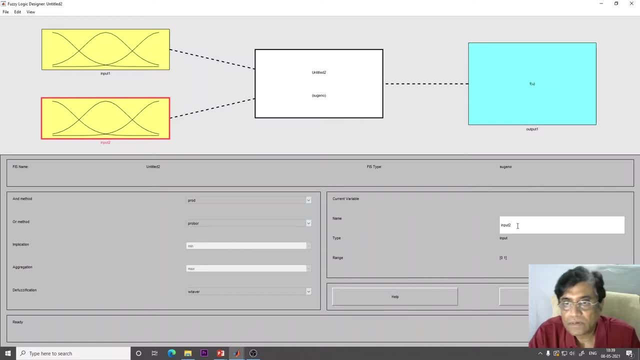 will use to import one. so say level of art and then say, okay, these are my. so you see, this cell has given you input output internally. now I can just configure it to solve my problem and then output. no, Welcome output. right, so I will satisfy people now. 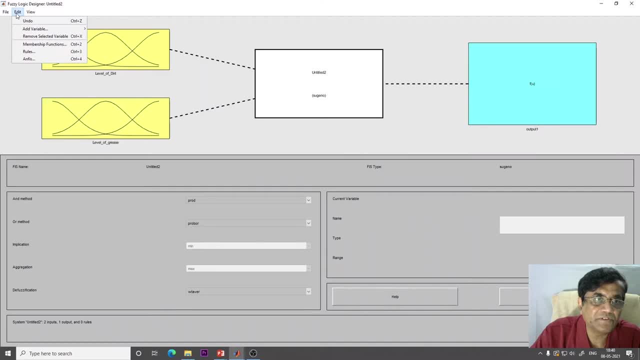 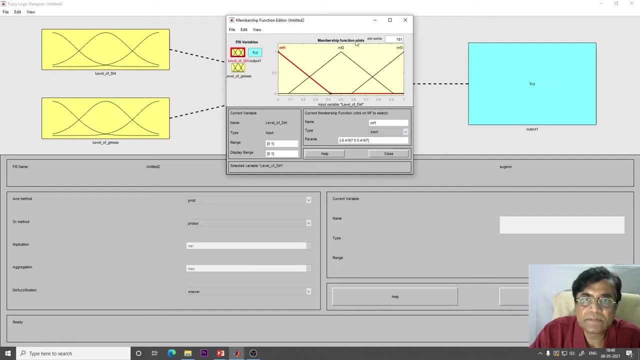 what we'll have to do. we'll have to add a membership function right. so now, as for You see, this is the level of dart See membership function by default it is there. Say: I will tell this membership function I am remarketing for, say, low, low dart, less or less. 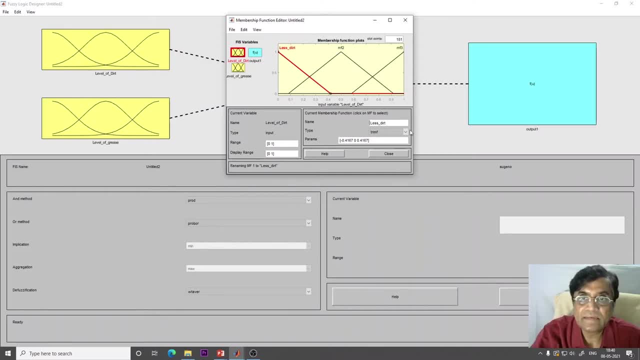 Less dart And say I have by default so many membership function. I am selecting this, So I am selecting right- Average, less dart- Okay, And say my membership is. let's say less dart- Okay, And say less average height, High level of dart- Okay, And say okay. so this is my one input. Another input: similarly, I will have to do less, say less average height. 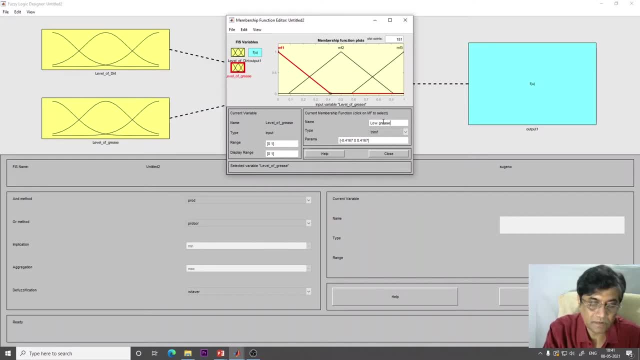 Low, Okay, Low. And then I have say decided Let's say, okay, average, See, I am just selecting average, low, all kind of fuzzy thing. But actual result which I will give, I will get, is not fuzzy. 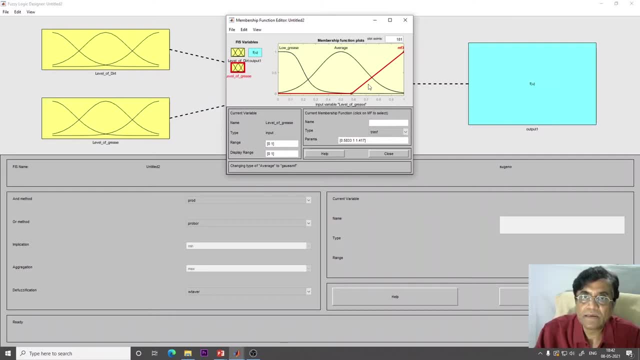 Low grease, Average grease level, And then let me see Average, Okay, And then this is say height: Okay, So now output- I will have to do. Okay, So now output, I will have to do. 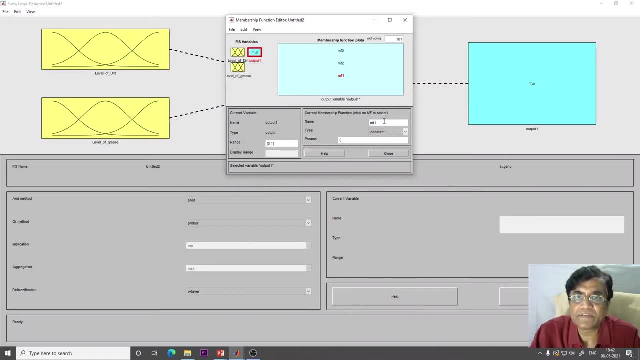 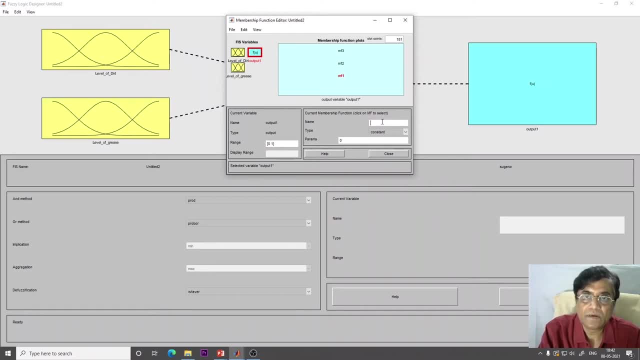 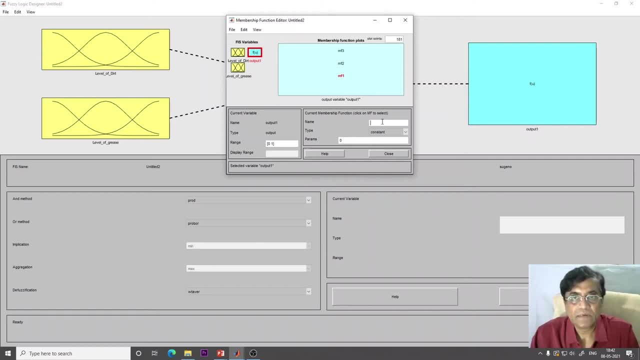 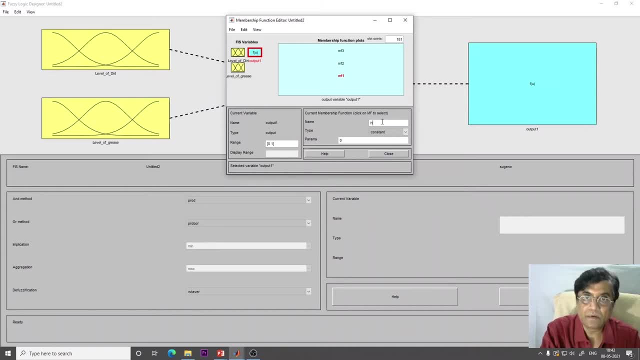 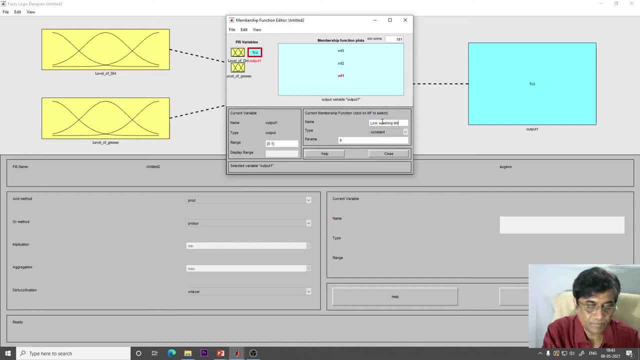 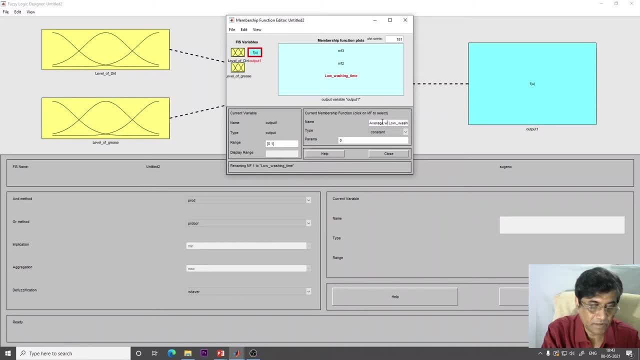 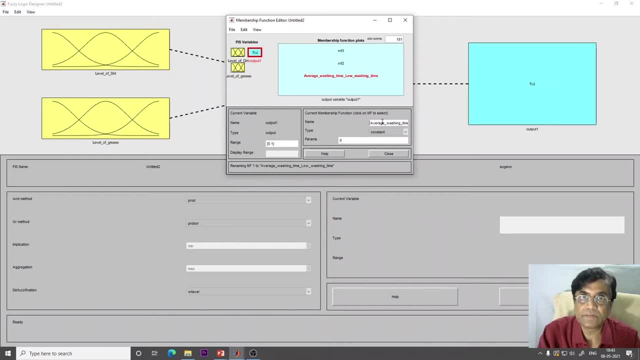 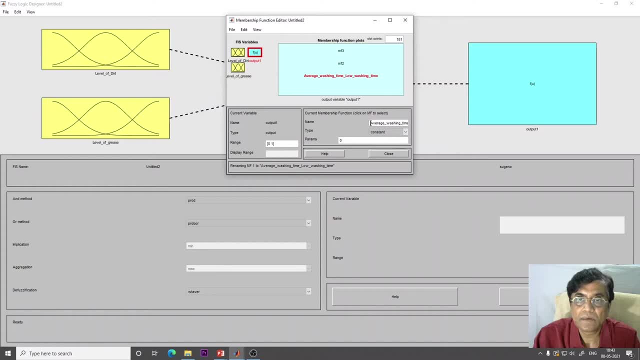 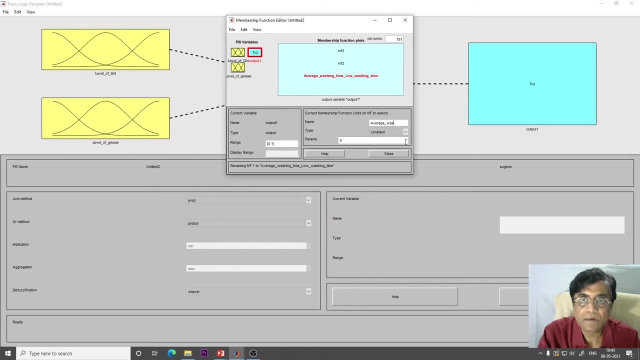 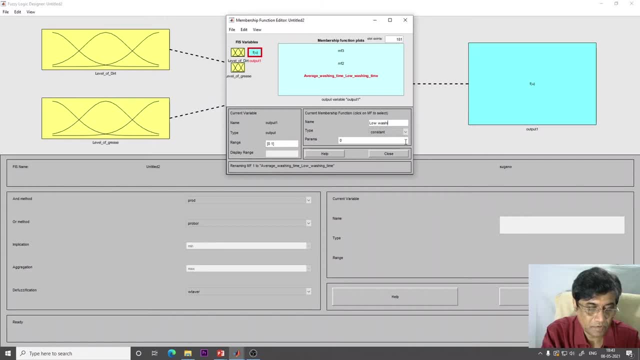 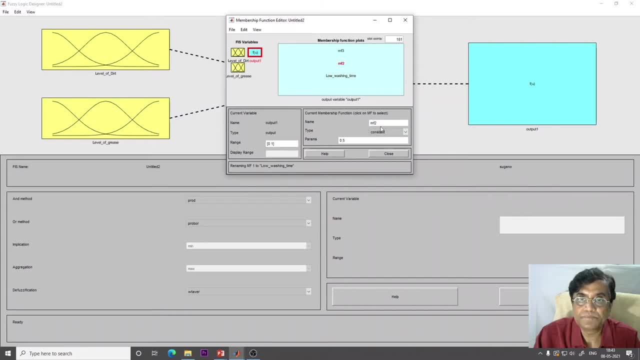 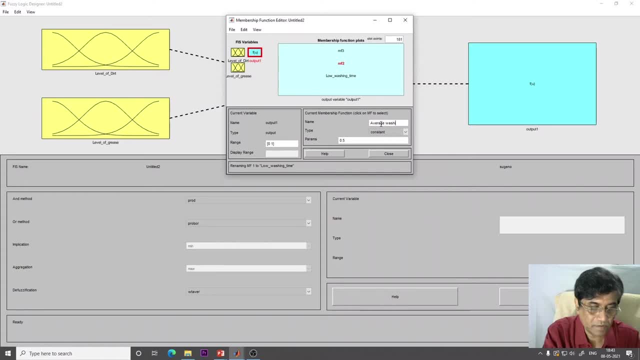 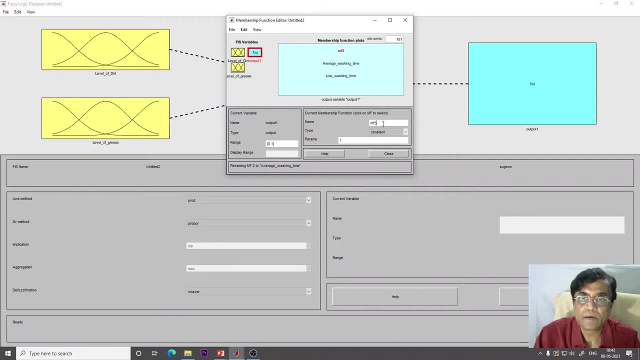 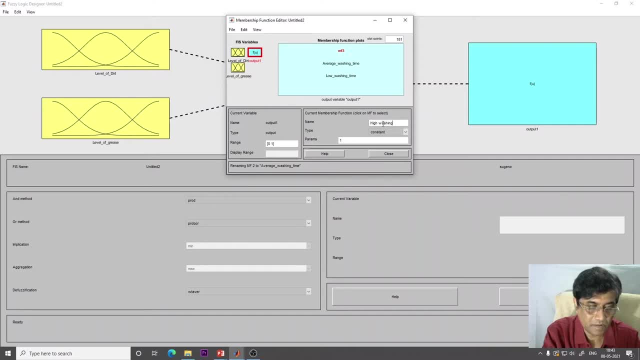 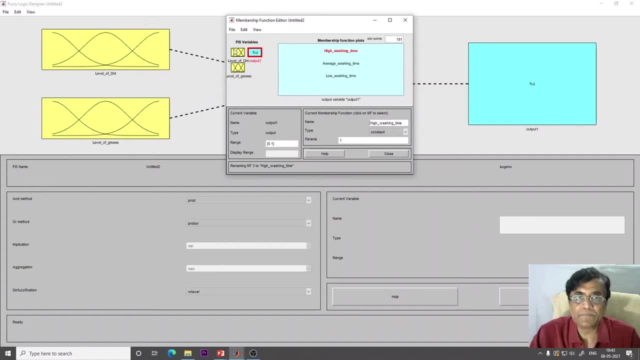 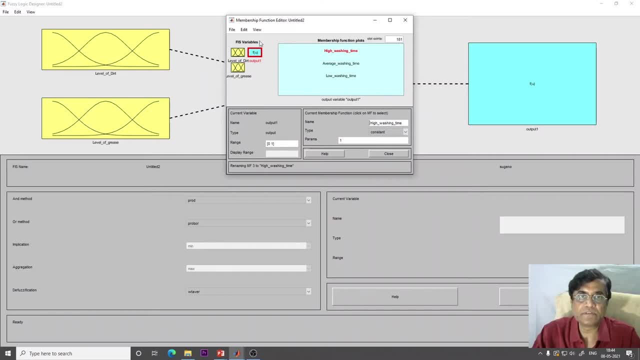 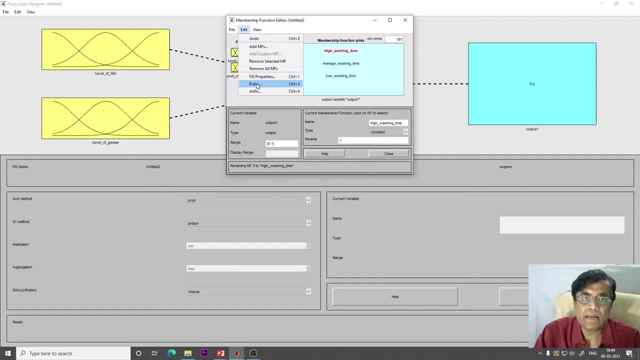 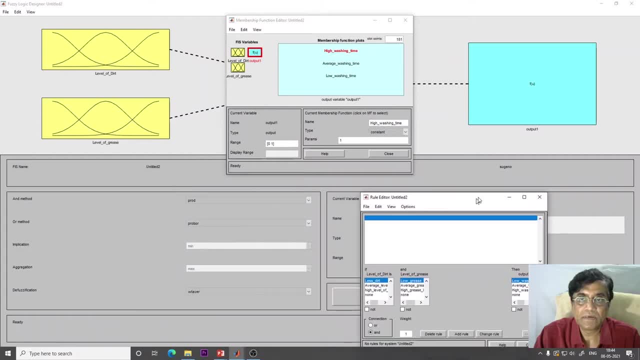 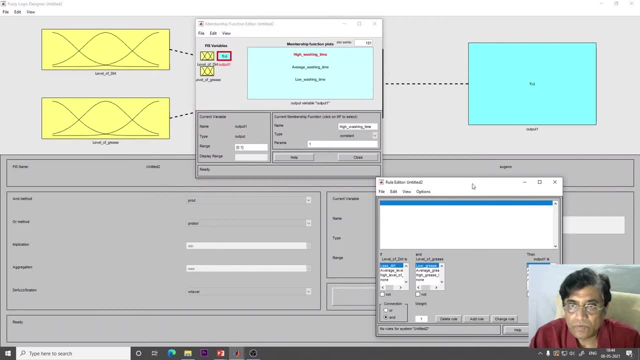 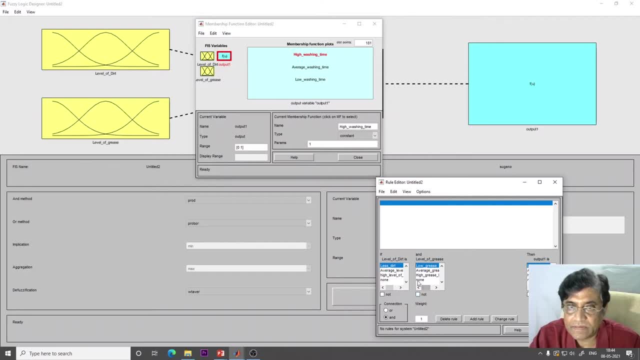 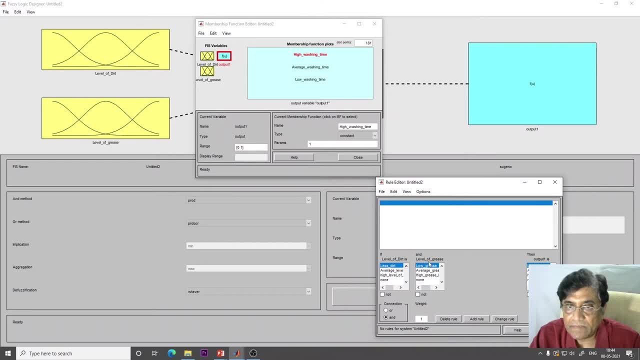 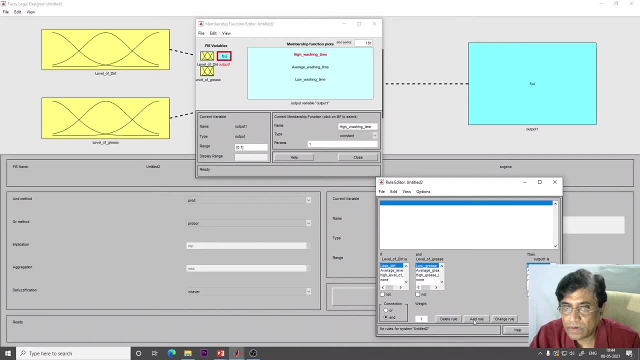 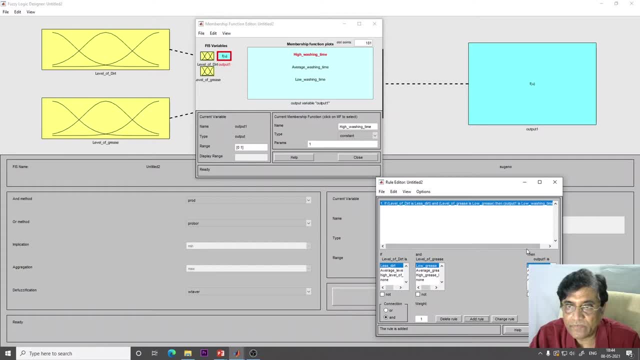 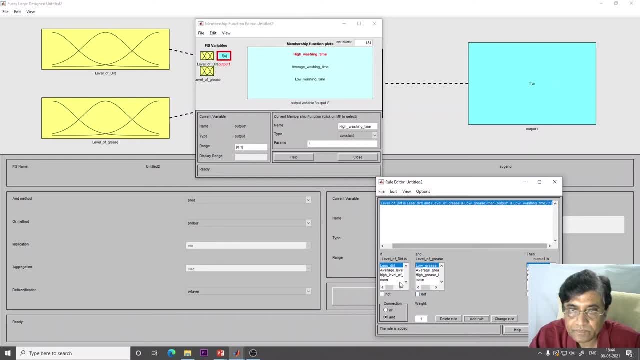 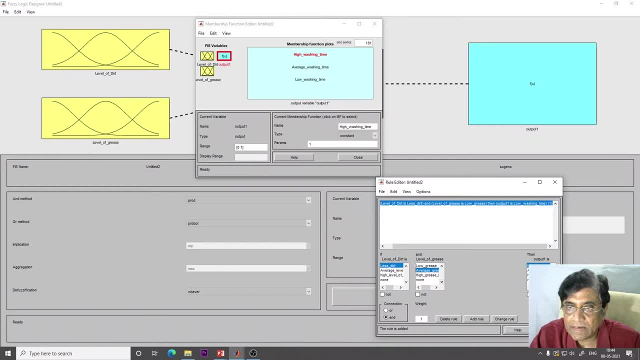 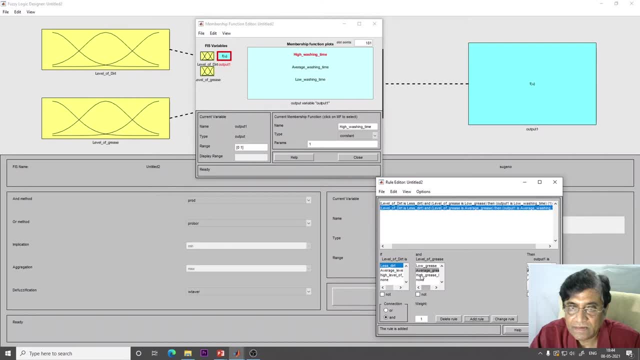 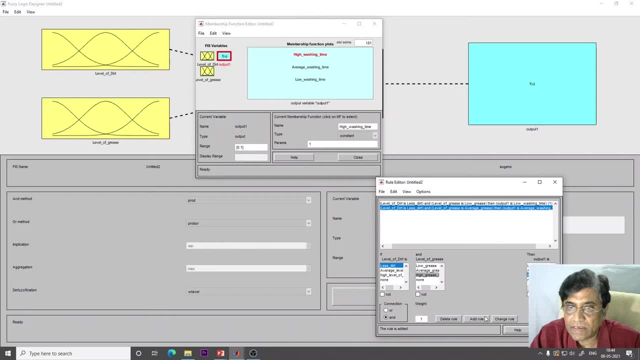 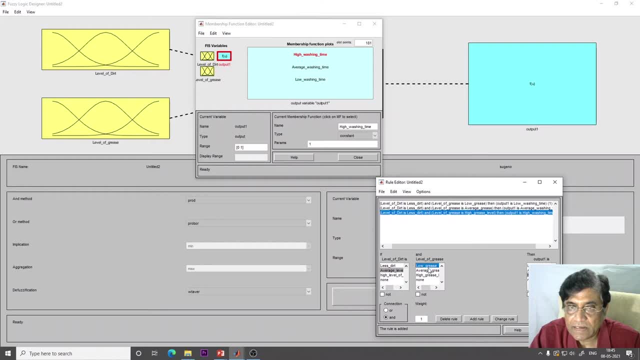 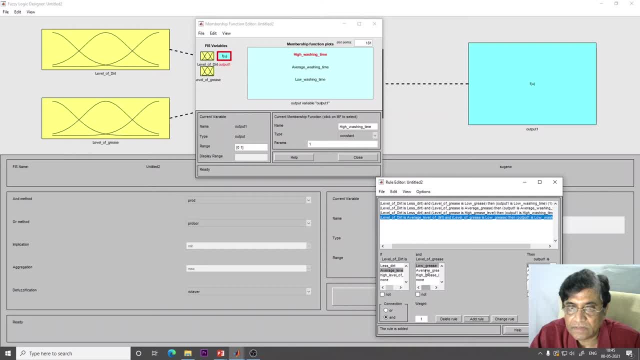 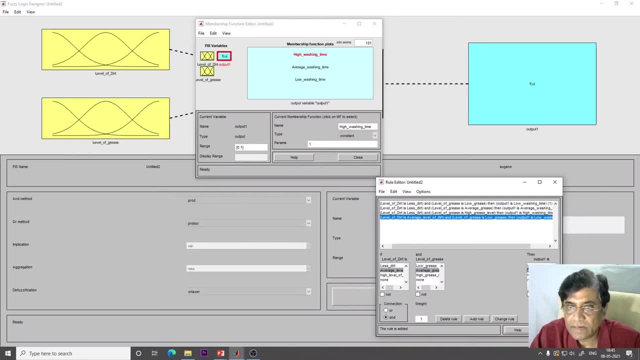 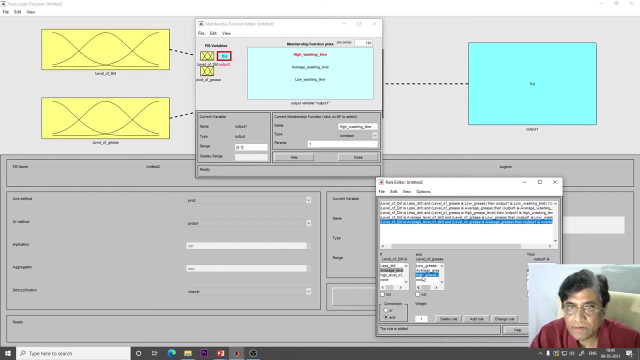 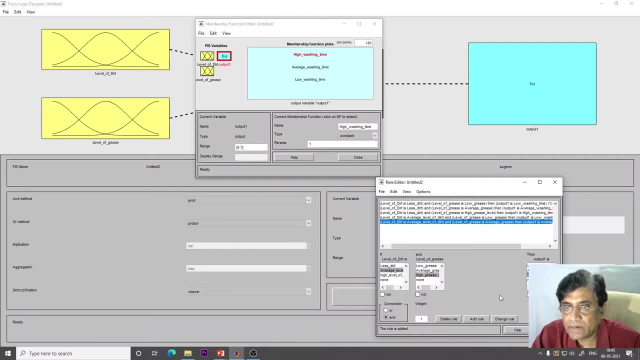 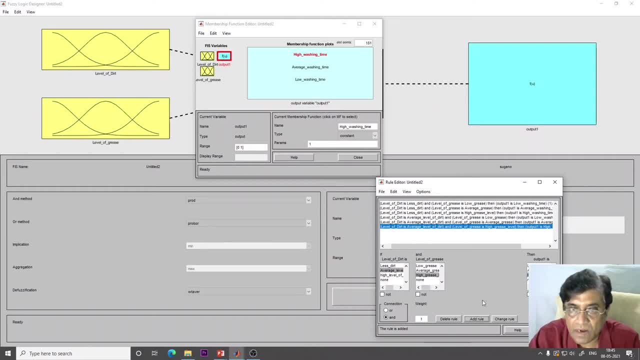 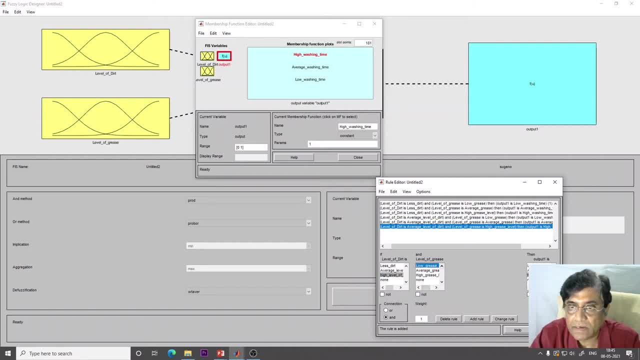 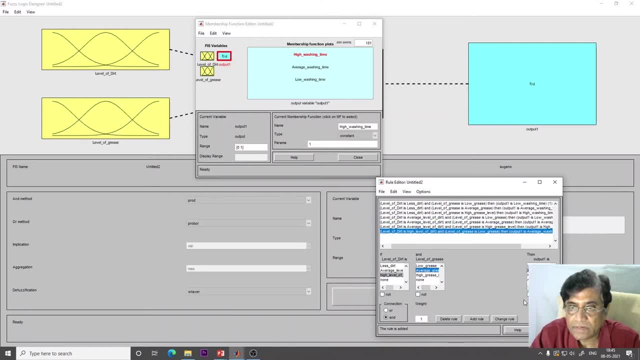 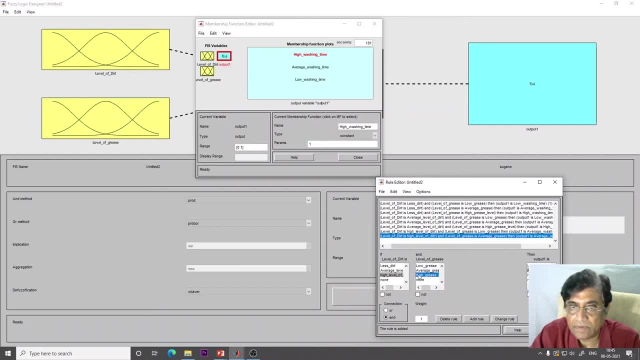 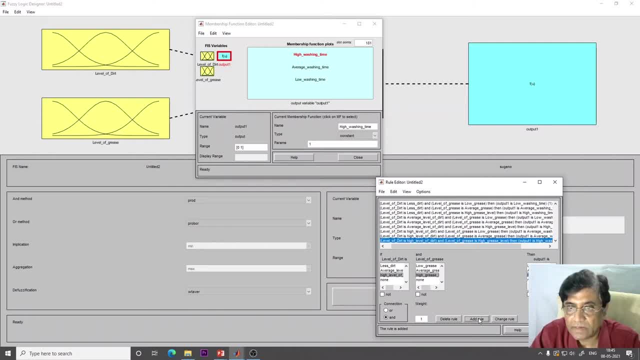 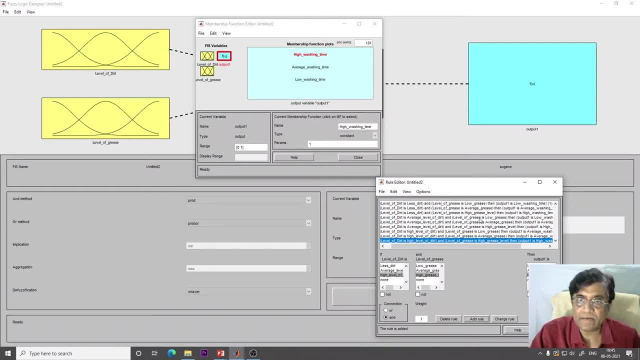 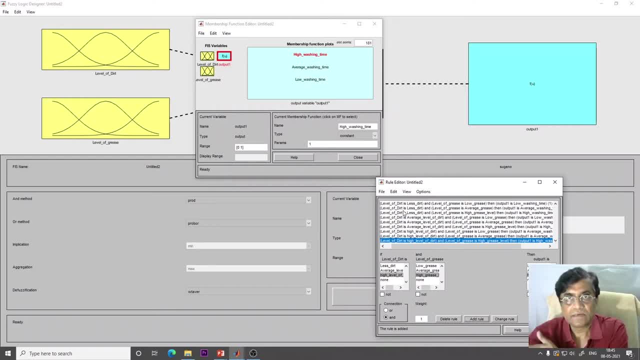 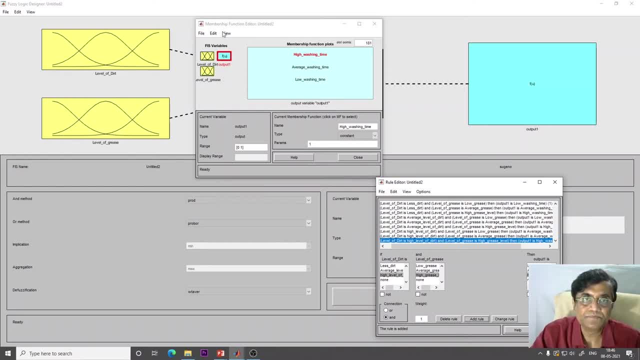 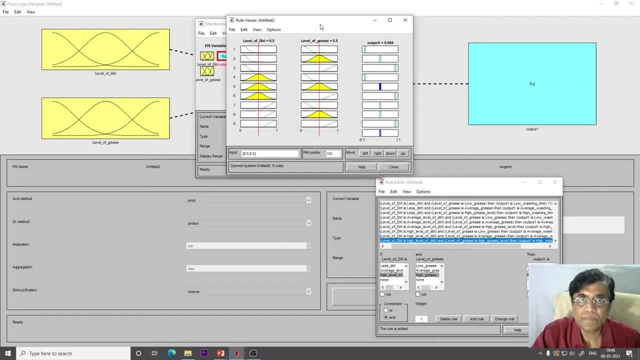 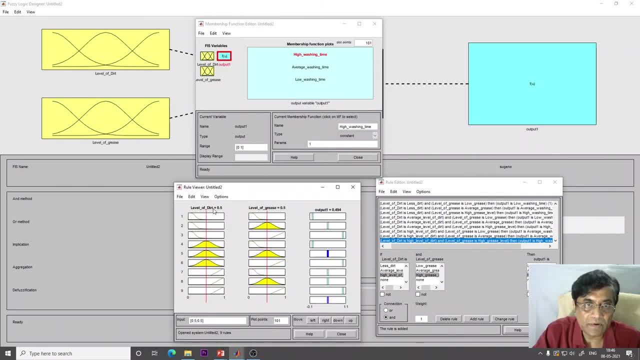 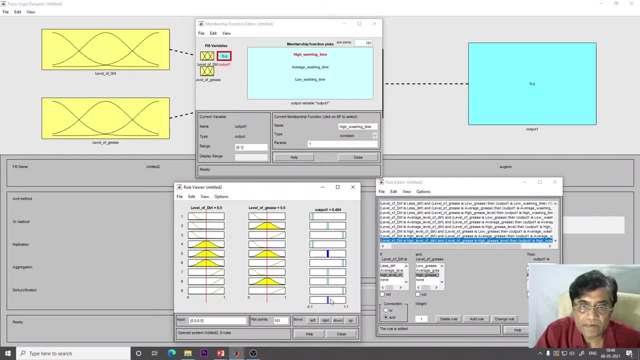 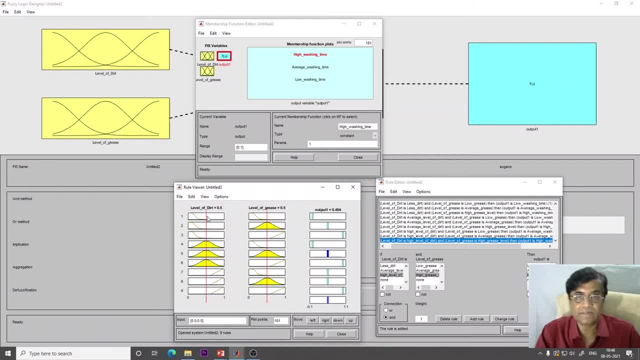 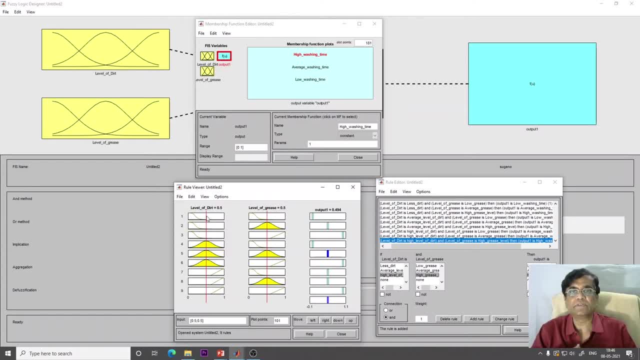 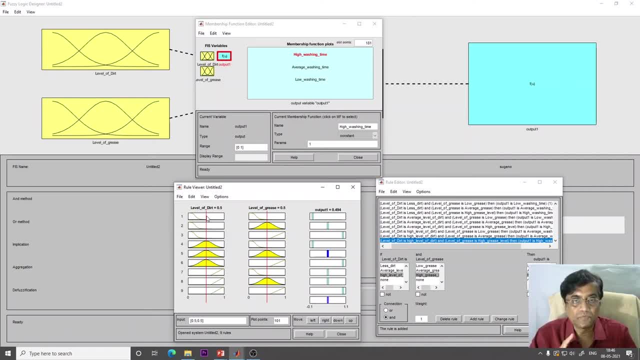 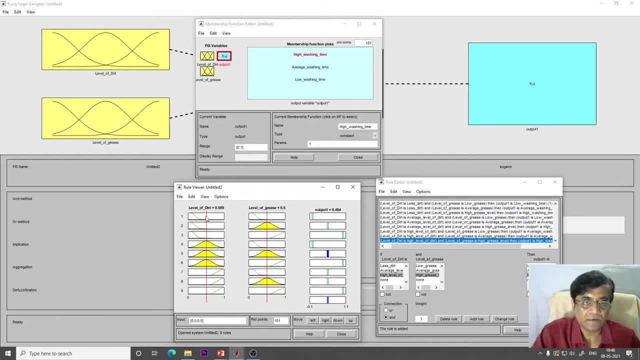 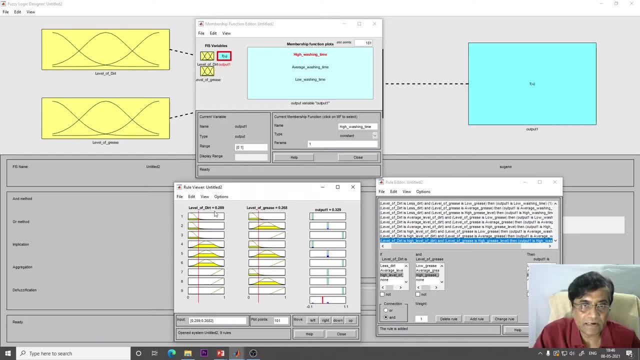 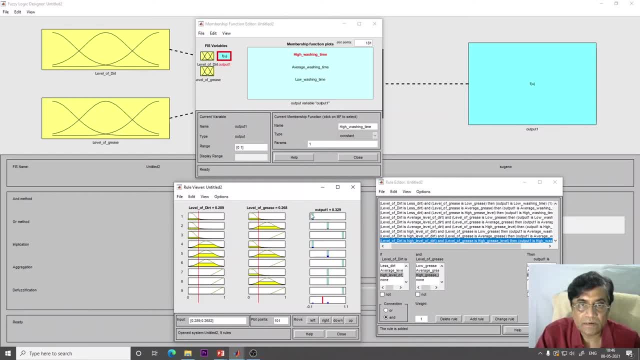 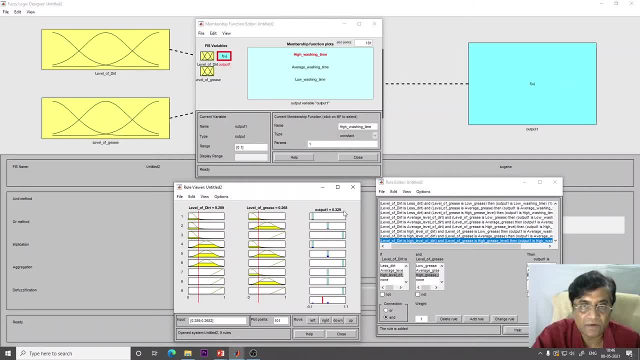 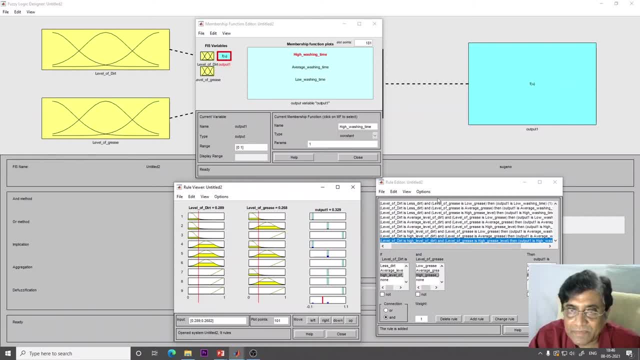 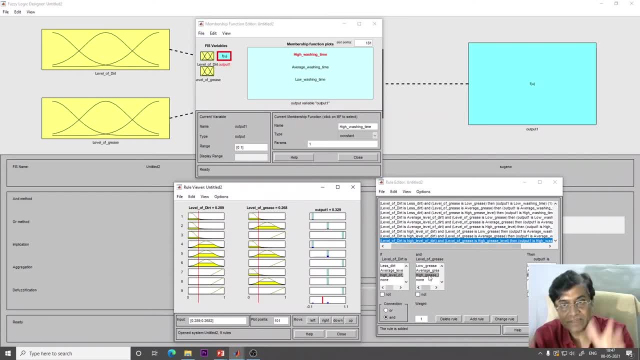 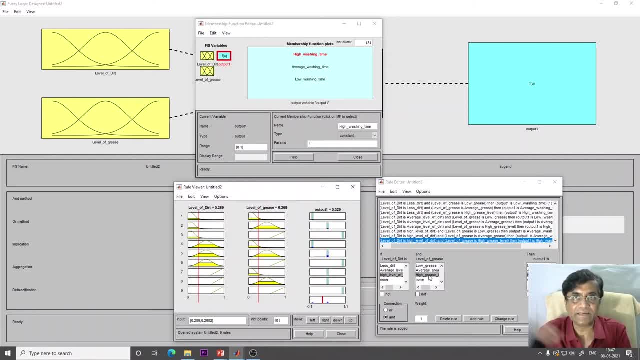 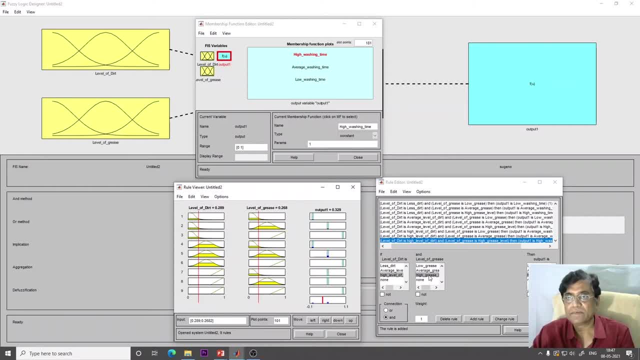 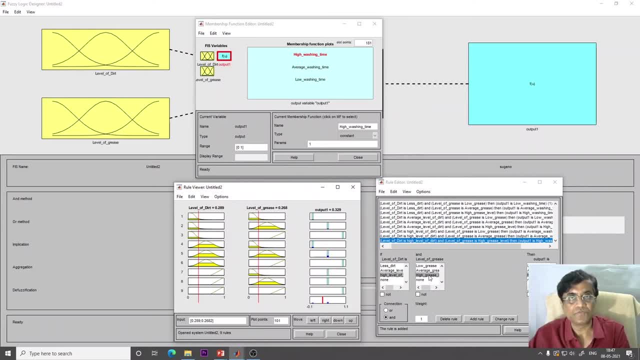 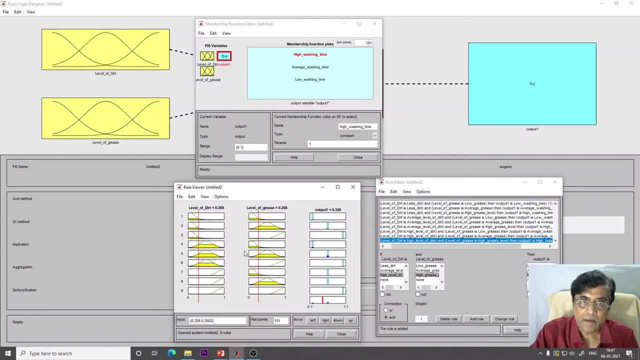 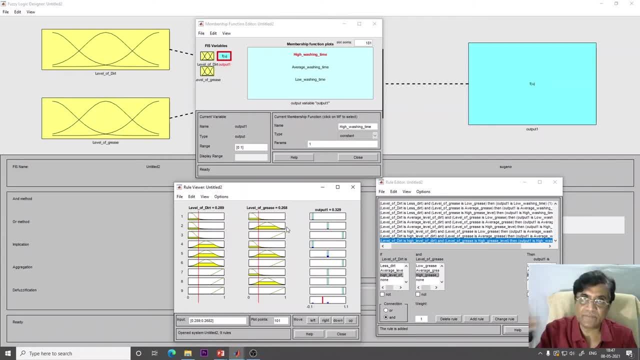 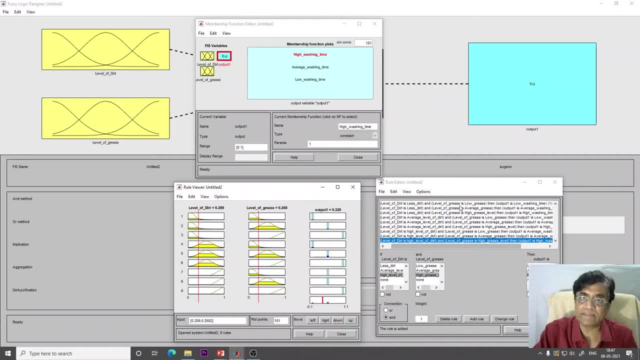 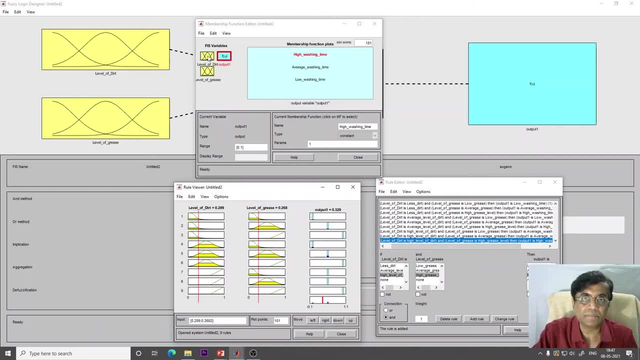 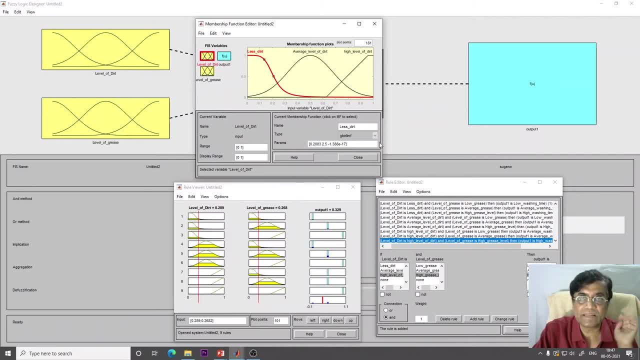 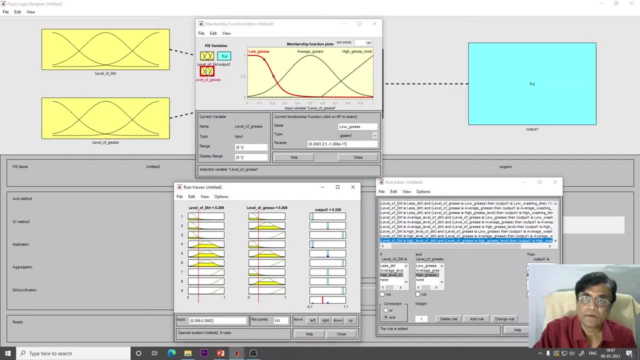 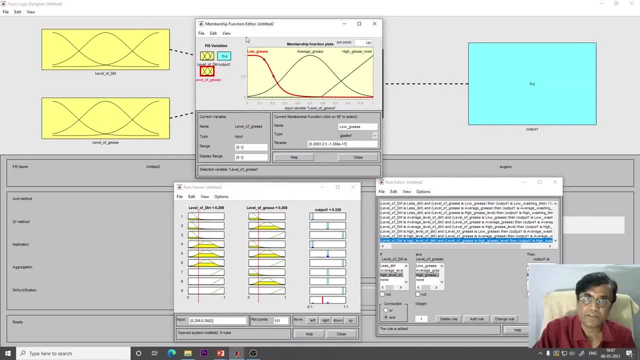 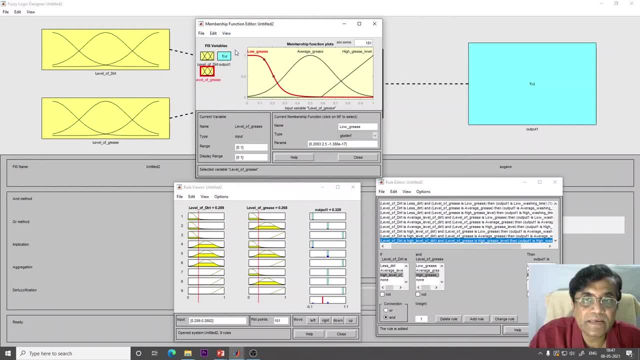 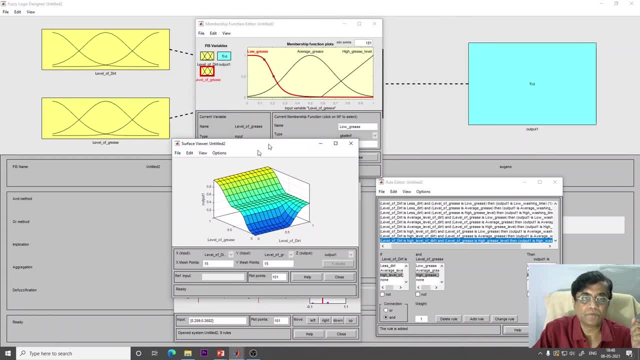 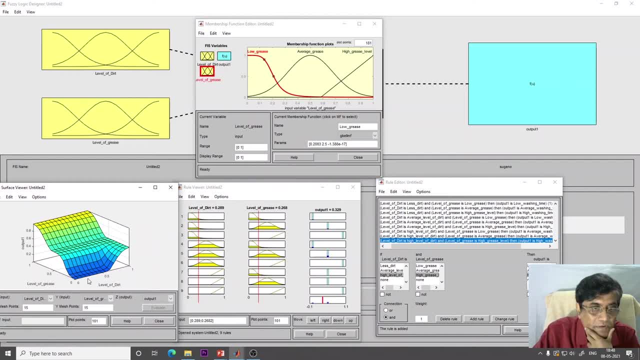 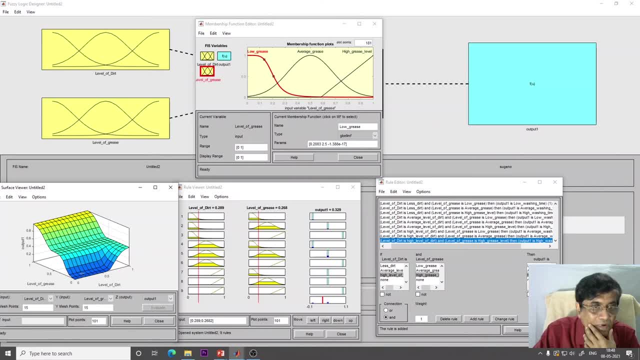 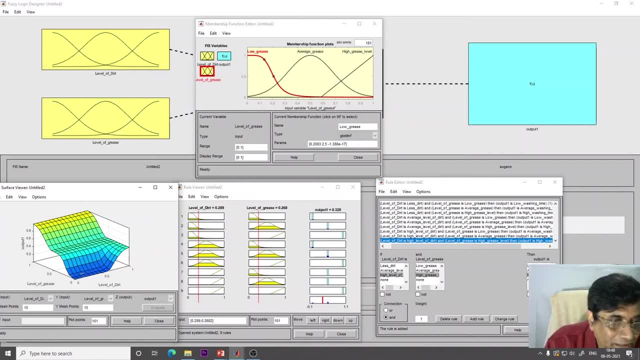 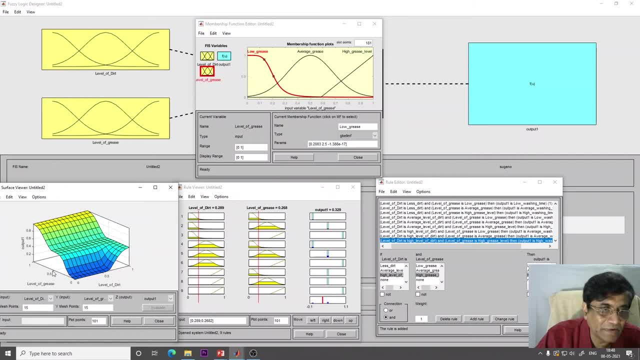 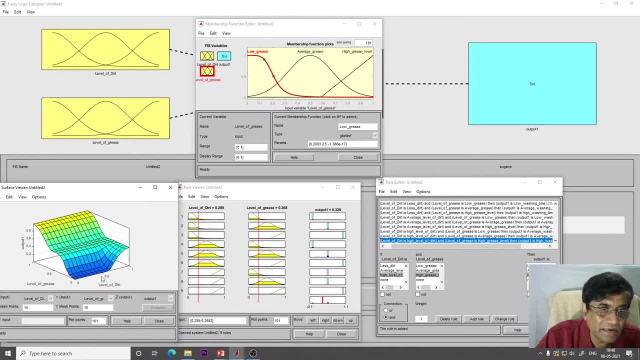 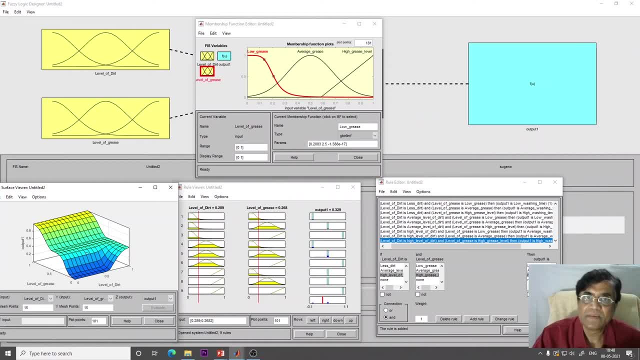 Okay, So now output. I will have to do hired time. so, basically, design is more or less correct, but you need to find you and lot of laborious thing you need to do. you need to just spend several hour time in consulting the expert and getting your past data to fine-tune all these things. that, what would be the most. 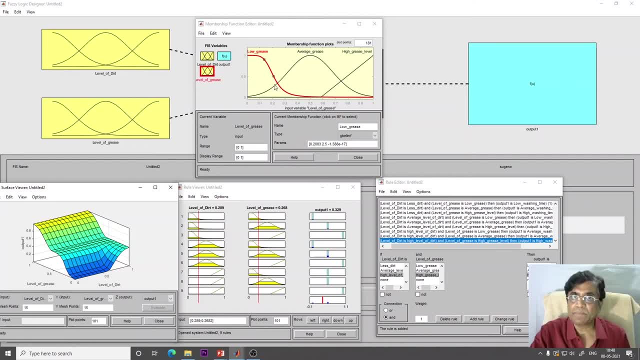 suitable membership function. what will be the rules i should uh incorporate? so you should uh do them correct. after several iteration, you fix the design. now, once the design is fixed, you got the data right. so this data, actually in the form of exam rule, you have written in the form of lookup table, those data will be stored in a fuzzy chip. so that chip, which